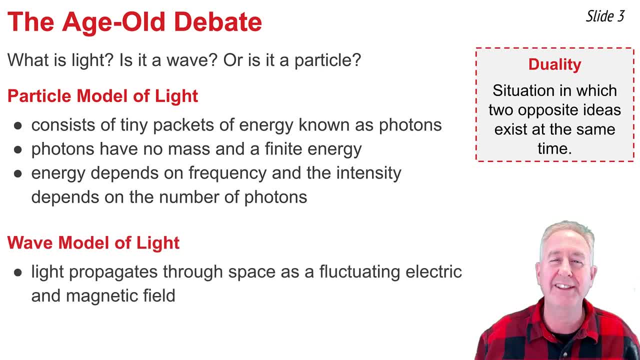 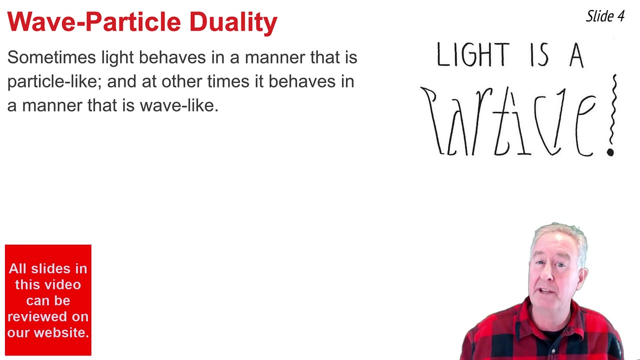 In contrast, the wave model of light suggests that light propagates through space as a wave with a fluctuating electric and magnetic field. Such an electromagnetic wave has a varying wavelength and frequency and exhibits classic light. In contrast, the어가 quantum systems are wahrscheinlich cytерш lebby for the first place, ever moreys the. 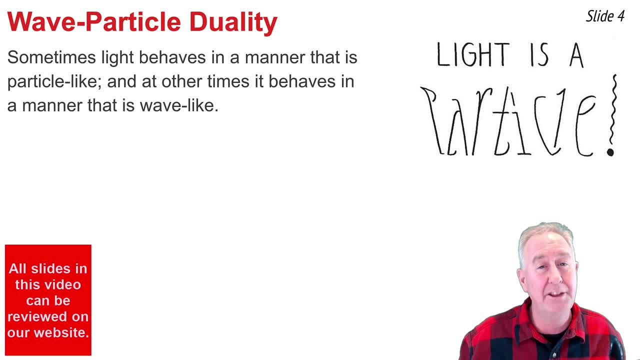 at times observe it behaving as a particle, and at other times you can observe light behaving as a wave, as the image above me indicates. you can look at the same thing, lightилаγ and edit. you can observe both particle and wave. This idea of wave particle duality is not restricted to light at all, but instead you have light movement and thus both particles. This idea of wave particle duality is not restricted to light at all, but instead maioria粒 ane to aspect dimension sch— away from the infinite range of you and me around, which might carry the amount of light that you have, speech points and less sound energy. 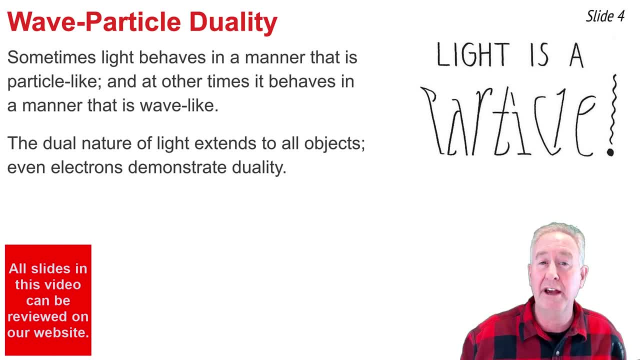 With soccer thousand foliougray on the fact that if you follow a quantum system, thes, whether acceptable, describes the whole of nature. There's considerable evidence of even an electron behaving as a particle and also behaving as a wave. So what are the behaviors of light that distinguish it from? 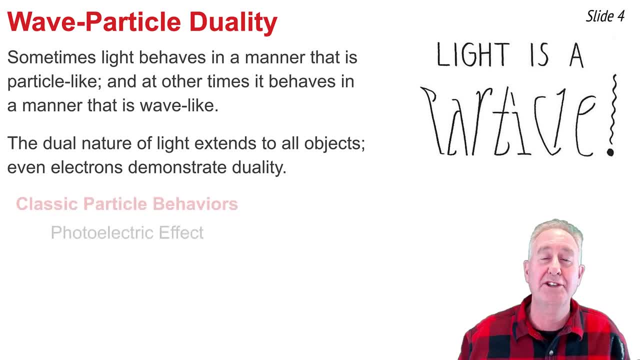 being a particle versus being a wave. The most classic particle behavior of light is the photoelectric effect. This is the effect that is observed when light strikes the surface of a metal and an electron is ejected from the surface of that metal. The actual kinetic energy of the 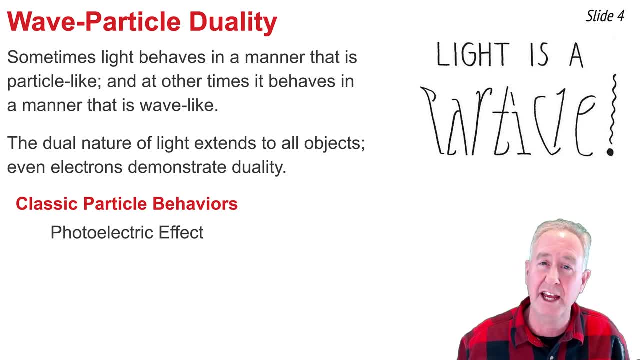 ejected electron is dependent upon the frequency of the light. Increasing the frequency increases the kinetic energy of the ejected electron, but increasing the number of photons that strike the surface has no effect upon the kinetic energy of the ejected electron. This is an observation that is contrary to the wave model of light and supports the particle model. 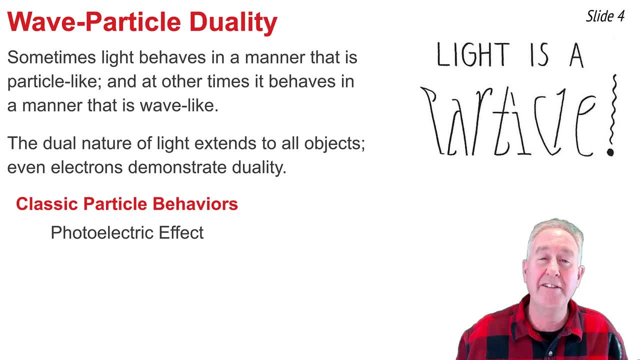 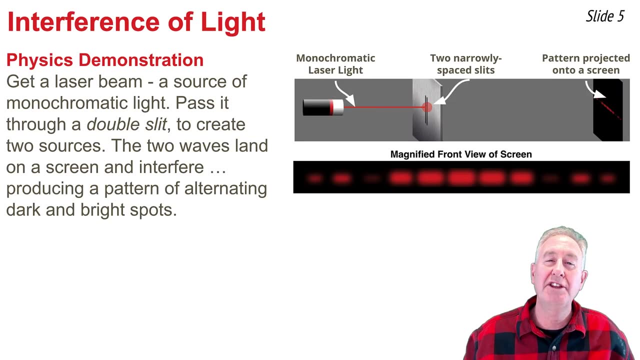 The three behaviors of light that support the wave model are interference, diffraction and polarization. Since this entire tutorial series is upon light waves in color, we'll be spending more time discussing these three wave behaviors. Perhaps you've seen the demonstration in which red laser light is shined up on a double slit upon a slide. The light passes through the 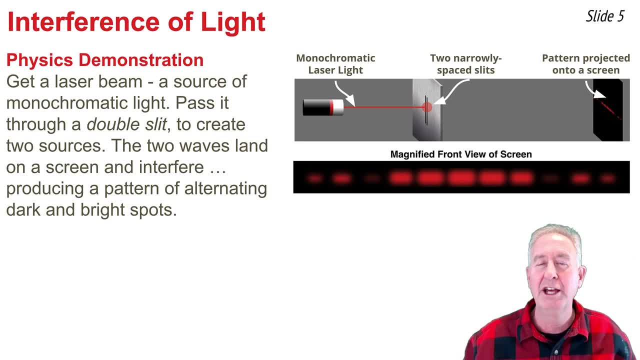 double slit, thus forming two sources of red light which are then projected on a double slit. The light passes through the double slit, thus forming two sources of red light up onto a screen within a dark room. Upon the screen, you observe a pattern of alternating. 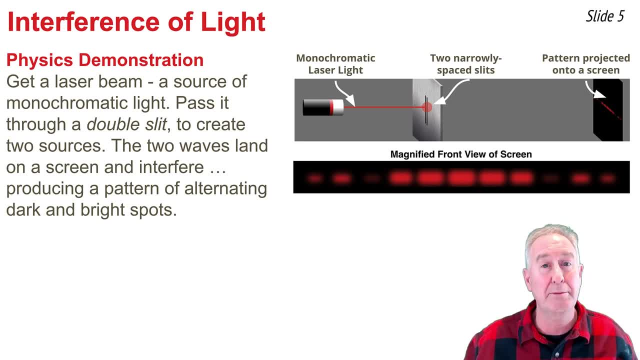 dark and bright red bands. The dark points upon the screen are locations where light from the two sources have landed and destructively interfered to cancel each other out, resulting in darkness. But the bright red bands upon the screen are locations where light from the two 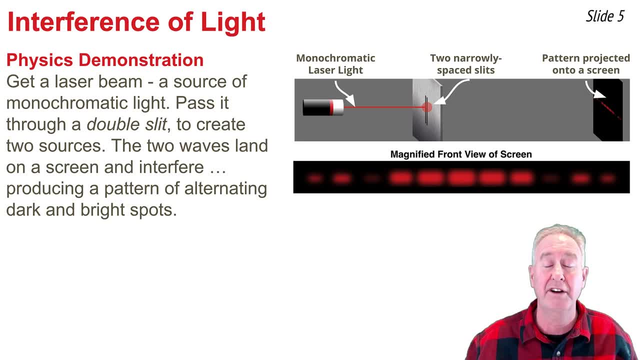 sources have landed on the screen and constructively interfered, thus producing a location of maximum brightness. An experiment like this, without a laser, was performed by Thomas Young in 1801 to provide evidence that light undergoes interference and thus behaves as a wave. 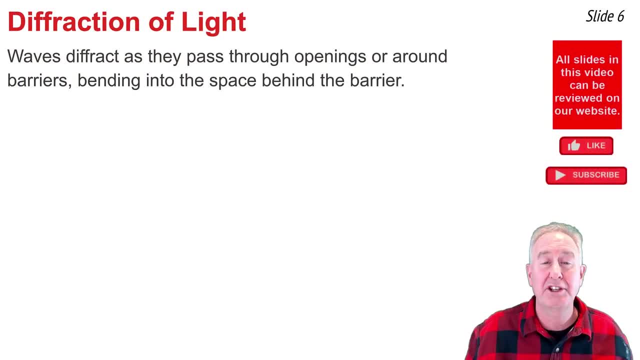 Diffraction is a well-known wave behavior. Diffraction describes the tendency of a wave to pass through an opening or around a barrier and to fill in the region of space directly behind that barrier. This diagram illustrates the way water waves traveling through a tank and approaching an 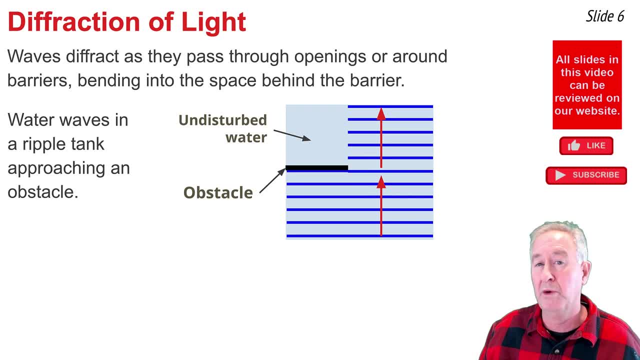 obstacle that is in its path. The diagram shows the waves reaching the obstacle and continuing straight ahead. The region directly behind the obstacle is water that is undisturbed, But this is not what happens, What really happens when we observe water waves approaching an obstacle. 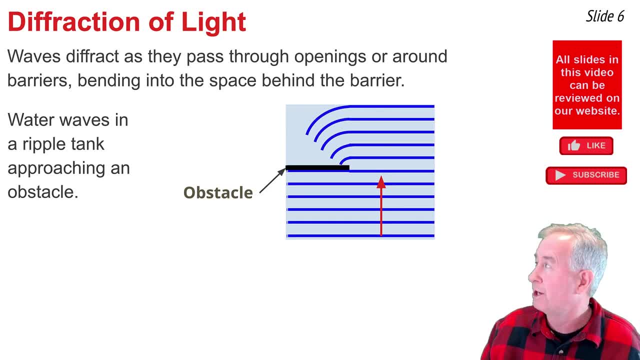 is. we observe it bending into the region of space directly behind the obstacle. We would observe small ripples within the water behind the obstacle, indicating that water is not disturbed by the waves, but that water waves are undergoing diffraction. The tendency of a water wave to undergo 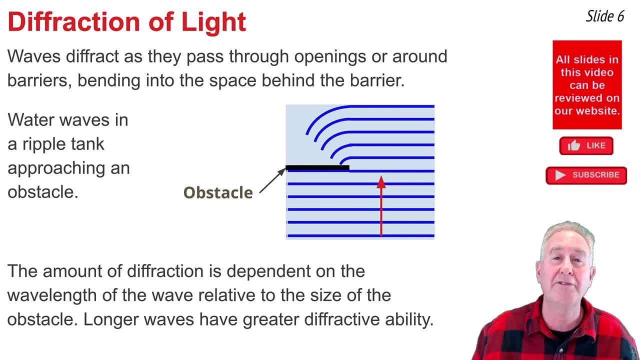 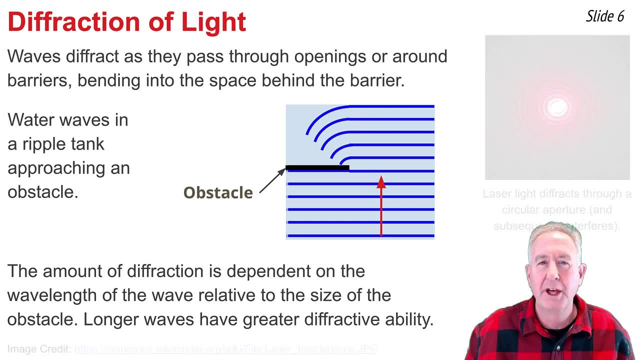 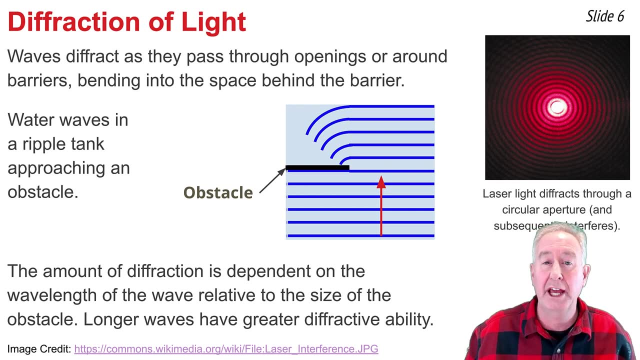 diffraction depends upon the wavelength of the waves relative to the size of the obstacle, with longer wavelength waves undergoing a greater amount of diffraction. The photograph above illustrates the result of shining red laser light upon the eye of a needle. The laser light will pass through the 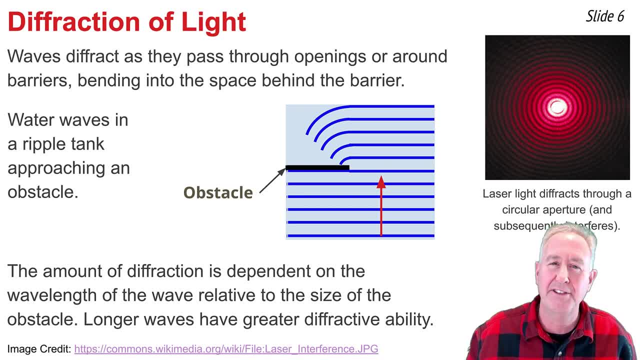 opening of the needle and also around the edges of the eye of the needle, and then undergo interference. The laser light will then pass on its way to a screen. Upon the screen, we see an interference pattern that results from the diffraction of light both through the eye of the needle and around the eye of the needle. 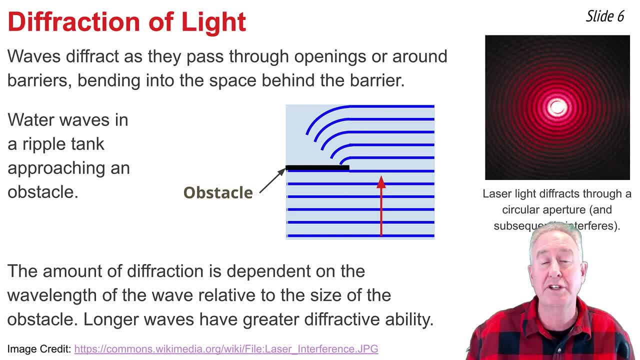 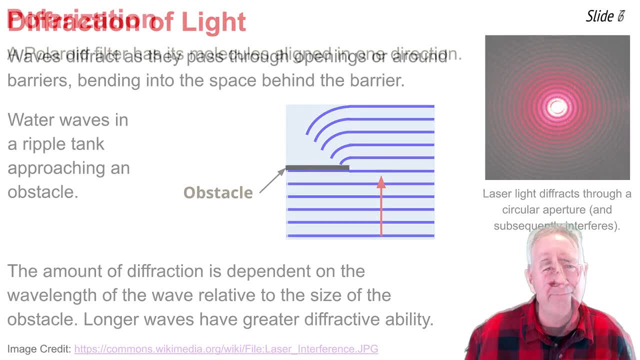 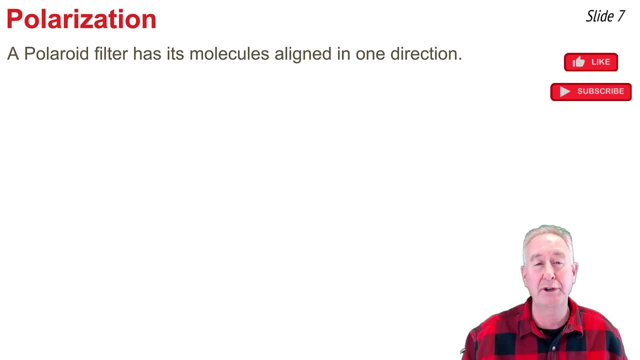 These two behaviors, diffraction and interference, are characteristic of all waves, and this demonstration provides evidence that light has wave-light behaviors. Polarization is a third behavior of light that supports the wave model of light. A Polaroid filter is a manufactured material in which 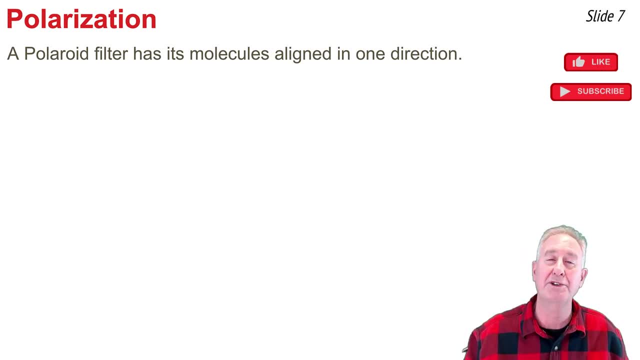 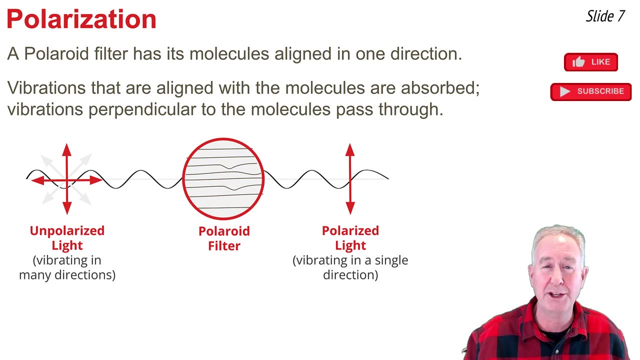 all, or a least most, of the molecules are aligned in the same direction. We can think of the vibration of light that are in the same direction as the molecules as being absorbed by the filter, while vibrations that are perpendicular to a molecule will pass through the filter. In a simplified model we can think sometimes. 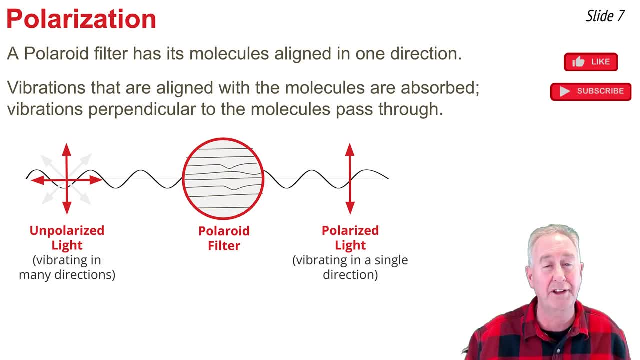 of light as having half of its vibrations going vertically and half of its vibrations going horizontally. As such, light approaches a particular light cheese and generation increases over time and therefore gives up. its light approaches a filter with the molecules aligned horizontally. the horizontal vibrations are absorbed by the filter and the vertical vibrations pass through the filter. 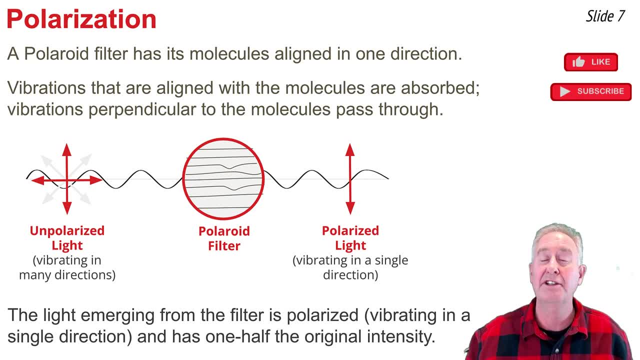 We would observe that the emerging light from the filter has one half the intensity as the original intensity and is vibrating in a single direction. If you were to take two Polaroid filters and align them such that their molecules were perpendicular to one another, then you would observe that the first filter would absorb. 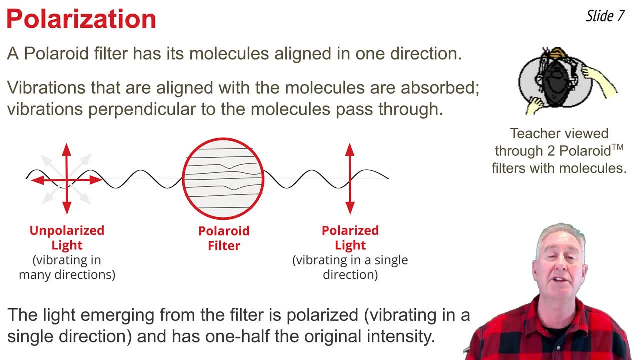 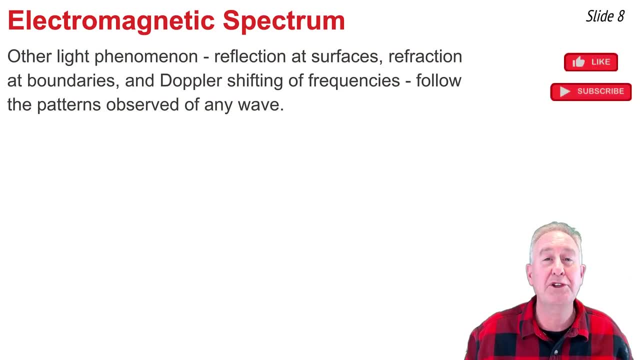 one half of the light and the second filter would absorb the second half of the light and no light would get through both filters. In addition to interference, diffraction and polarization, there are other behaviors of light, such as reflection at surfaces, refraction at boundaries and the Doppler. 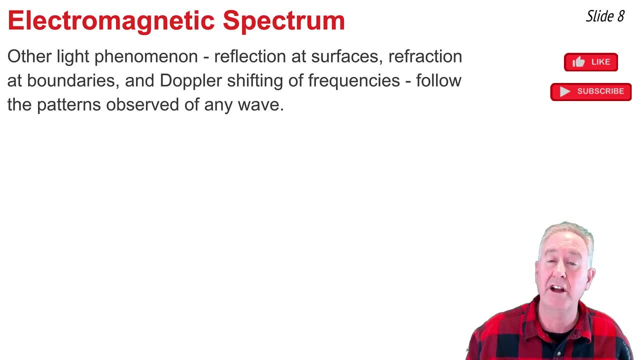 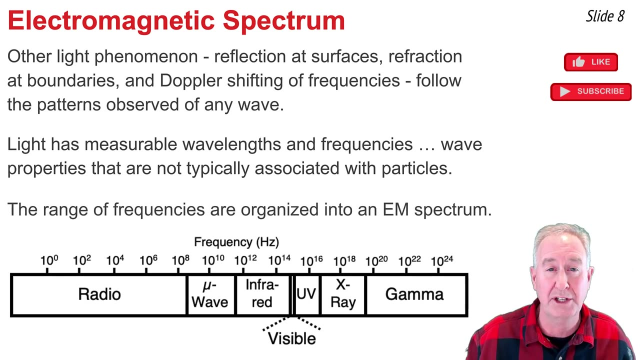 shifting of frequencies that follow the patterns observed of others. Furthermore, light has measurable wavelengths and frequencies. These are properties of waves that are not typically associated with particles. A matter of fact, the wide range of frequencies of electromagnetic waves are typically organized into an electromagnetic spectrum, something that you've likely encountered in other. 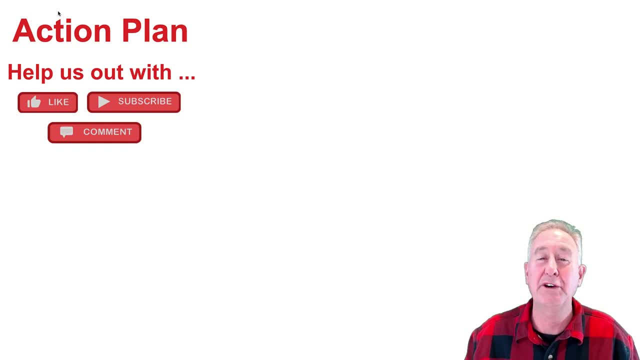 science classes. It's at this time, in every video, that I like to help you out with an action plan, a series of next steps for making your life easier. Thanks for watching, But before I help you out, could you help us out by giving us a like, subscribing to. 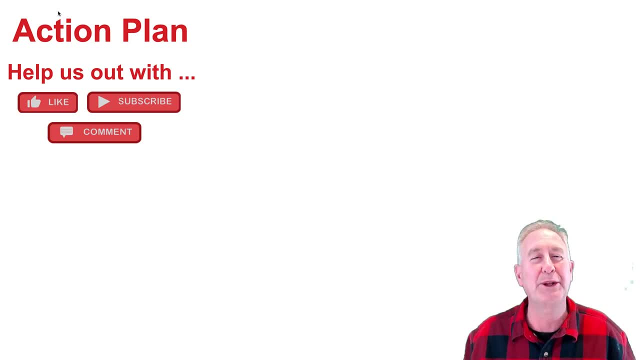 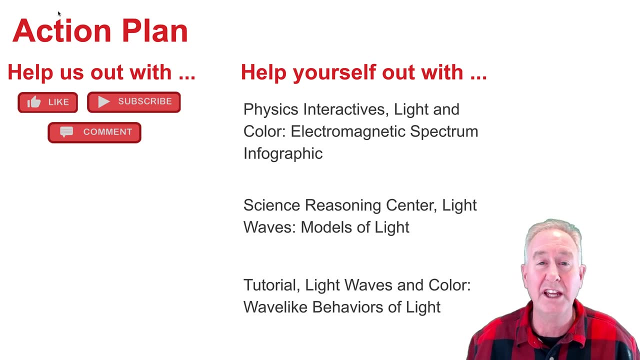 the channel or leaving a question or comment in the comments section below. Now for your action plan. Here are three resources that you'll find on our website, and I've left links to each in the description section of this video. We have a wonderful interactive infographic that is surely to amaze.